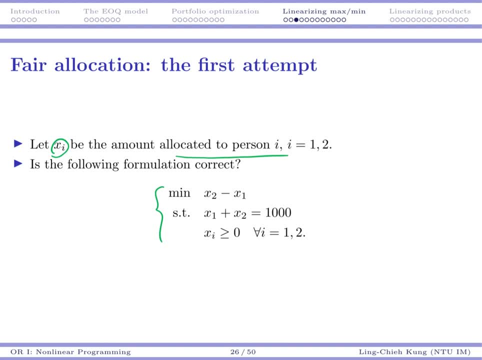 i would formulate this program. So when i do this, i want to minimize the difference subject to the sum would be 1,000. And that's all i have. But then if i do this, obviously this formulation is not correct. Why is that? Because with this formulation, 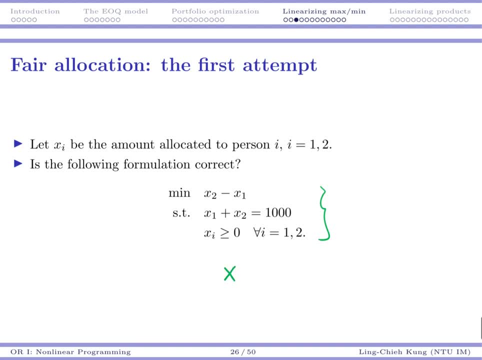 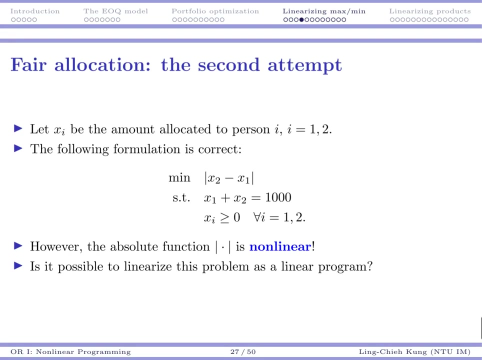 obviously my best solution is that x1 would be 1,000 and x2 would be zero. The difference goes to negative 1,000, which is optimal. But actually this is not fair at all right, Because the way we formulate the difference is not so good. What we actually should do is that we should. 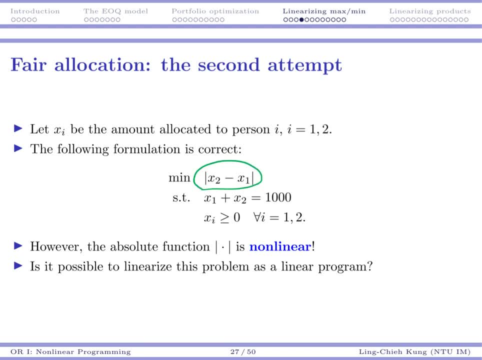 introduce, for example, the absolute function here. Okay, either x1 is greater than x2 or x2 is greater than x1.. We should always let the greater one to subtract the minus the smaller one, okay. So if that's the case, then this seems to be a much better formulation. 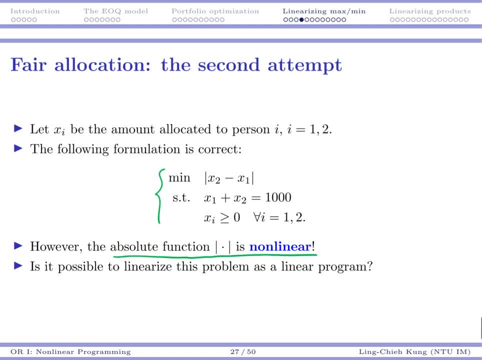 However, the absolute function is nonlinear. Why is that? Because pretty much it looks in this way: This is x, This is your absolute value of x. If you are having 5,, it goes to 5.. If you have negative 3,, it goes to 3, right, So your absolute. 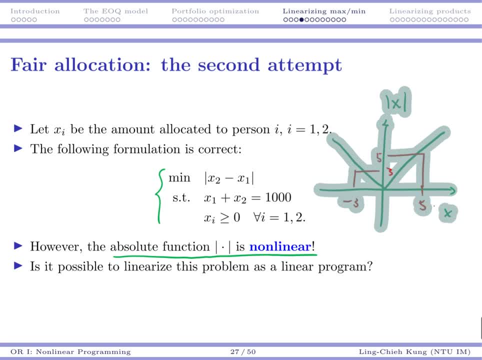 function. absolute value function is nonlinear, So we cannot just leave a nonlinear function here. That does not give us a linear program. We want to ask: is it possible to linearize the problem as a linear program? Of course there's a way, Otherwise it cannot be an example, right. 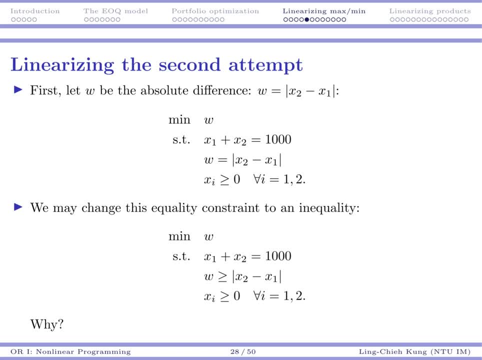 So let's see how to do this. So the first thing is that, okay, I don't like that absolute value function, So I'm going to replace it by another variable called w. So I now want to minimize w and I need to make sure that w is still equal to this absolute value of this difference. 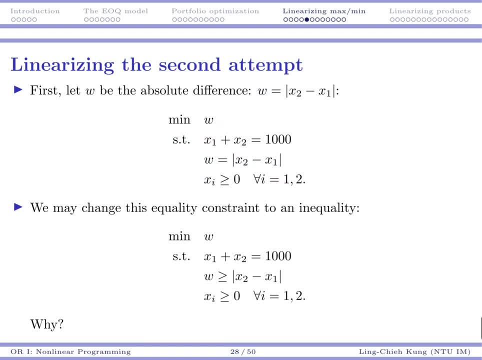 So, from here to here, actually, I didn't change anything. I simply call this difference, the absolute value of the difference, a name which is w. And then there's the key step. I'm going to argue that changing this equality to greater than or equal to does not change the. 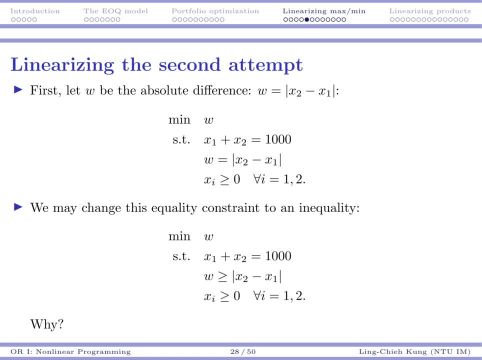 program. Well, let's see. why is that? Suppose we change this to greater than or equal to and we do some observation about this program, We would see that because we are minimizing w. okay, when we are minimizing w and w only appears in one constraint. 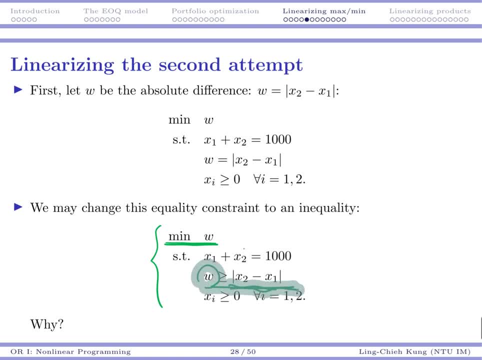 and w is lower bounded by the right-hand side, then in this case there must be- there cannot be no optimal solution where w is really greater than the right-hand side. okay, As long as this is true, it cannot be optimal. 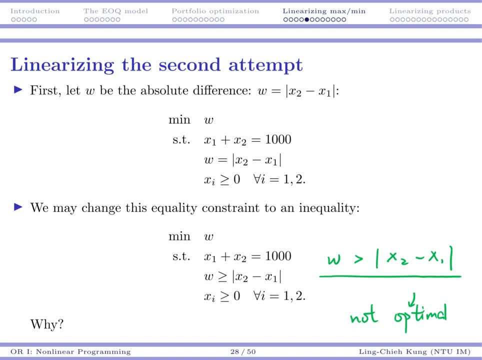 Well, why is that? Suppose you have an optimal solution saying that you have w, x1,, x2, and y1, and if it satisfies this particular strict inequality, then all you need to do is to further decrease w. There is a room right. So your original solution cannot be optimal. If you 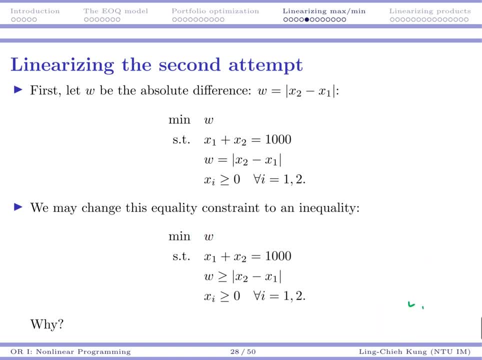 have an optimal solution. obviously, that optimal solution must make this inequality binding And if that's the case, it has nothing to do. it has nothing different from saying: an equality there, right? So the idea is important and the idea is simple. If you put it as an inequality. 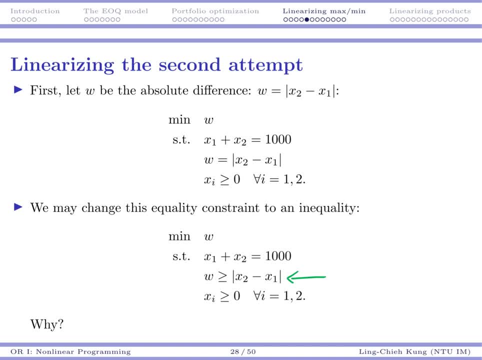 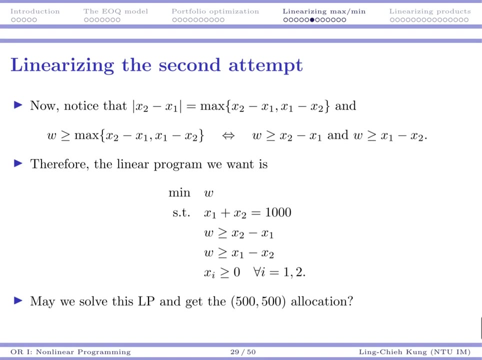 then at an optimal solution. this must be binding, so it doesn't really change your optimal solution From here to here. the feasible region, of course, is different, but the optimal solution is not changed. So now we also know that for this particular thing, the 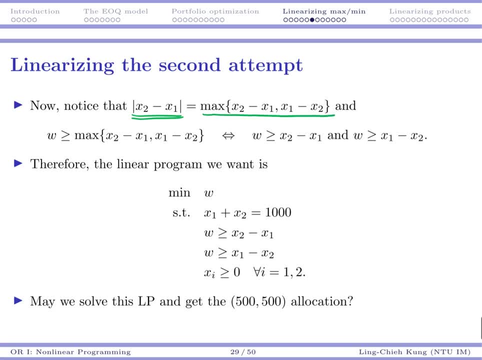 function can be expressed as the maximum of two things. So maybe you would like to review your graph. So this is x, this is square, This is the absolute value of x. Why do we say it is a maximum of two? Because pretty much this is your x, This is your negative x and your absolute value function. 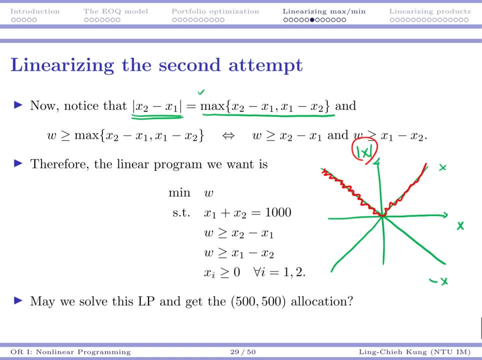 is this part? Does that make sense? So it's over. So with essa query we can ultimately необходимо taking the maximum between the two functions. that's why it takes a maximum there. so suppose that's the case now, because we are talking about x2 minus x1. 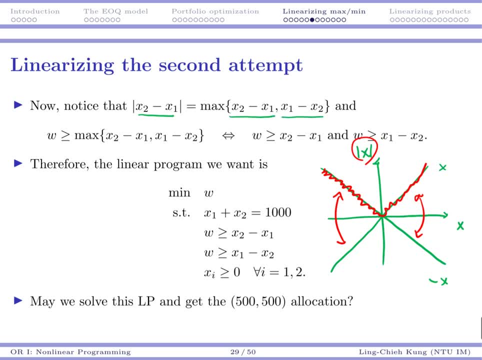 first we have x2 minus x1 and then we have x1 minus x2. the absolute value function is taking the maximum of these two makes sense. so if that's the case, then let's take a look at the formulation. pretty much we will say w. 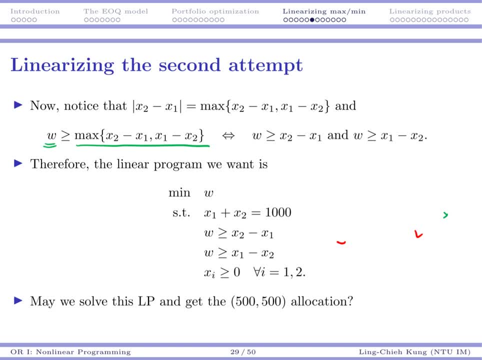 should be greater than or equal to the maximum of these two, then I actually can do this. I'm going to say then that means W should be greater than or equal to the first term and W should be greater than or equal to the second term. so suppose, 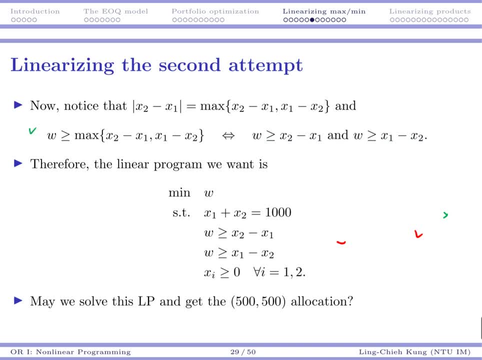 the left-hand side is true. in this case, your W is greater than the maximum of these two, then w naturally need to be greater than or equal to either one. if w is greater than or equal to either one, then of course w is greater than or equal to. 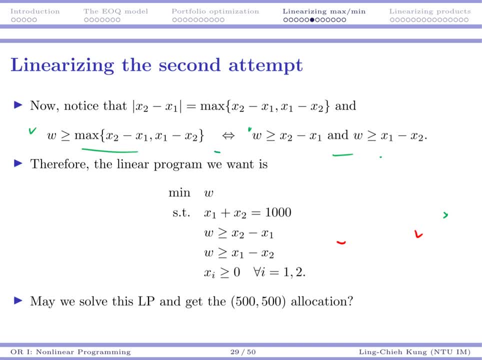 the maximum of these two. all right, so this is again something we can do. so now we finally reach a formulation with no maximum function or no absolute value function. all we need to say is that we want to minimize w such that w is either greater than, or w is greater than or equal to x2. 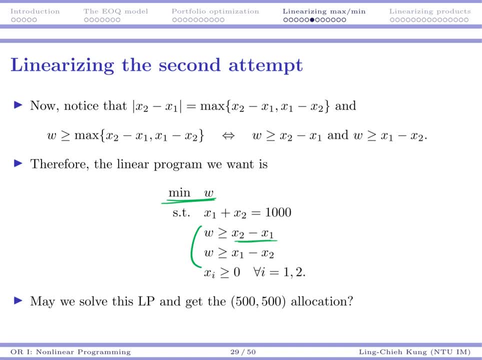 minus x1, and w is greater than or equal to x1 minus x2. so somehow one of them would be greater and then w would be lower. bounded by that greater amount, w becomes the absolute value of that two amounts. that's how the formulation makes sense. so, lastly, 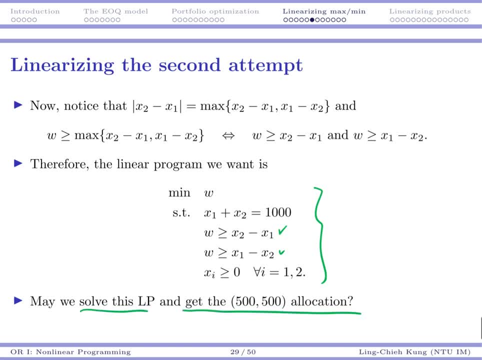 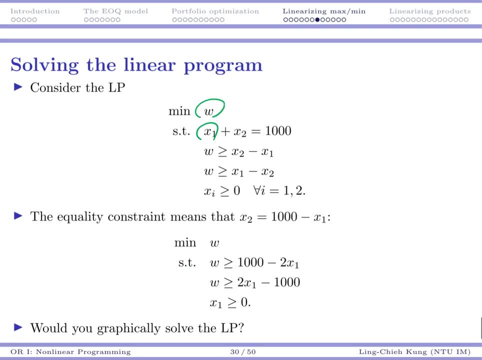 you can see that we have a formula for the absolute value of x1 minus x2. maybe we may try to solve this lp and really show you we would get a one half, one half allocation. well, that's not too hard. you have one, two, three decision variables, but actually you have an. 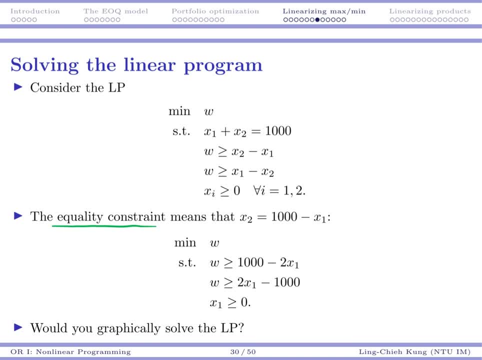 equality constraint that always allows you to remove one variable, for example x2. so we're going to replace x2 by 1000 minus x1. then our formulation becomes this one: now maybe we may use graphical approach to solve this problem. so let's say i have x1. let's say i have w, so x1 must be non-negative.